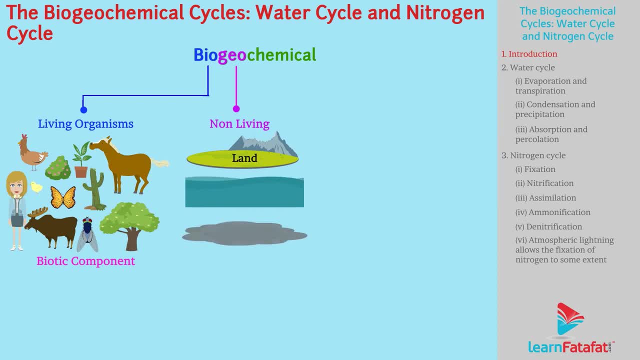 Geo suggests all non-living part of earth, like land, air, water. that is abiotic component, And chemical suggests different reactions occurring on earth. So what is biogeochemical cycle? It is the movement of chemical substances due to interaction of biotic and abiotic components of earth. 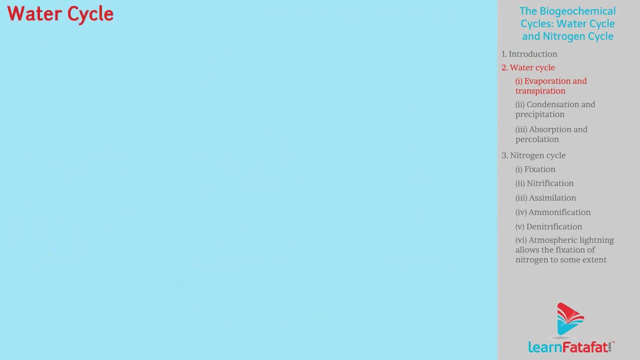 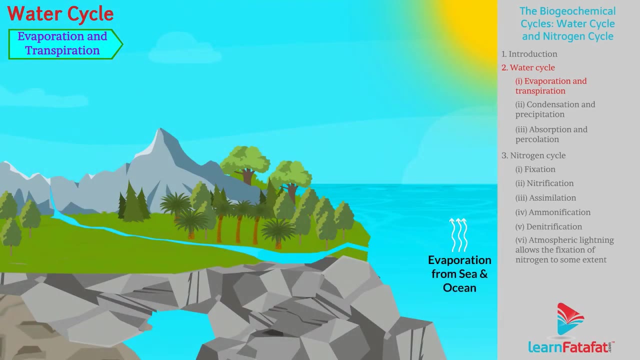 So let's start learning. water cycle, Evaporation and transpiration. Water from seas and oceans evaporates. due to the heat of the sun, Water converts into vapors and reach high in the atmosphere. Excess of water from plants undergoes transpiration. 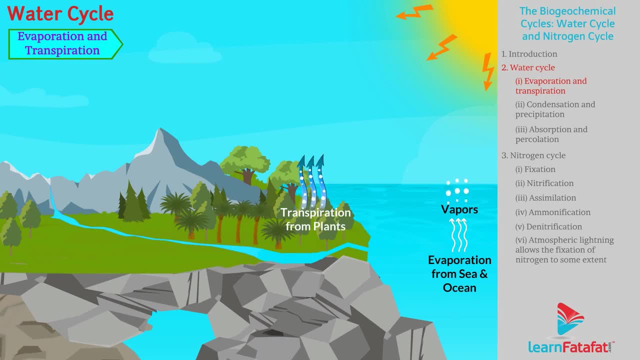 That is, water is released out of plant body in the form of vapors, Condensation and precipitation. Vapors reaching high in the atmosphere undergo condensation and turns into water droplets. These water droplets collect together and makes a cloud. Clouds are also carried from one place to another. 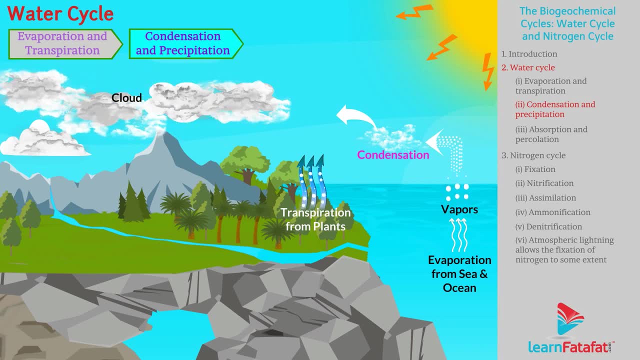 When cloud become heavy, it fall down in the form of rain. In condition of lower temperature, precipitation occurs and water drops freeze. In such case, there occurs snowfall or hailstones. Absorption and percolation: Water falling on the ground get absorbed into ground. 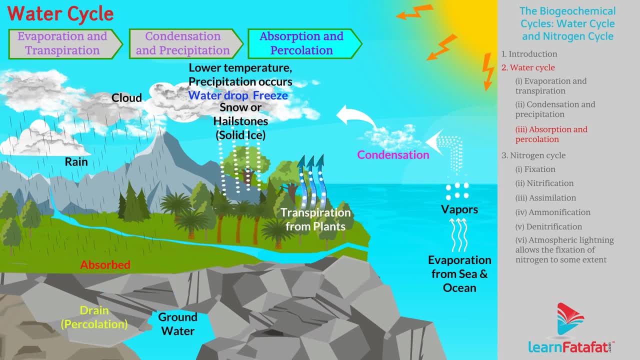 This water gets drained into the soil. Water running through the rocks and meets the ground water. Water running off from the hills meets the flowing water And the ground water, and flowing water somewhere meets the seas and oceans. This completes water cycle. In this way, water from sea and oceans returns back. 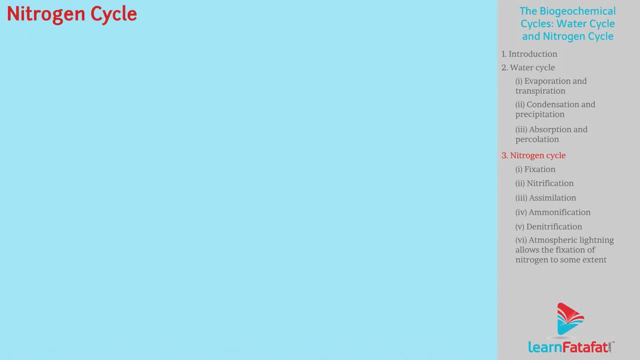 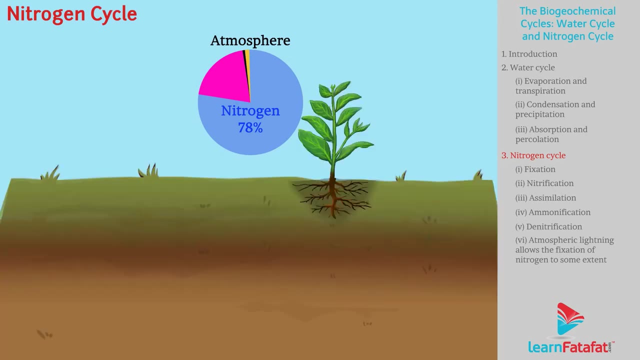 Nitrogen cycle- Nitrogen cycle For students. nitrogen occurs as 78% part of atmosphere. It is important part of life as it makes up proteins, nucleic acids, etc. The atmospheric nitrogen is difficult to use. Hence there is necessity to fix this nitrogen in its useful form.